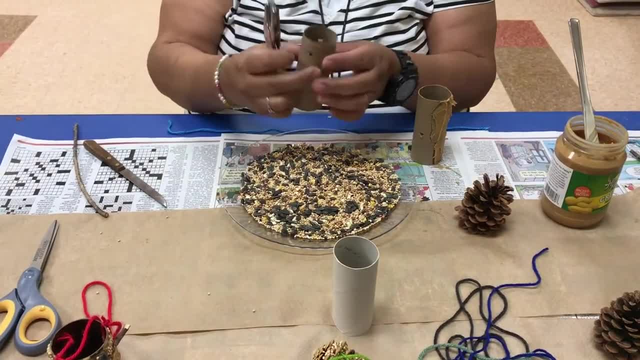 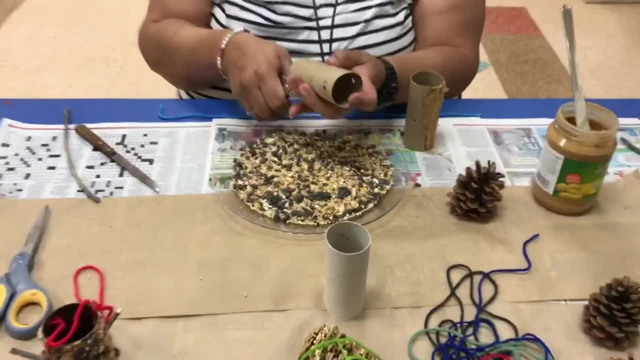 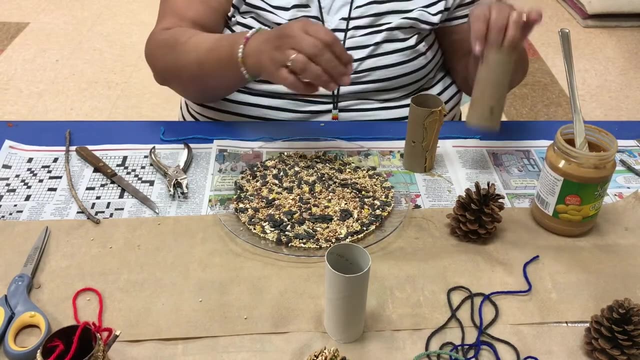 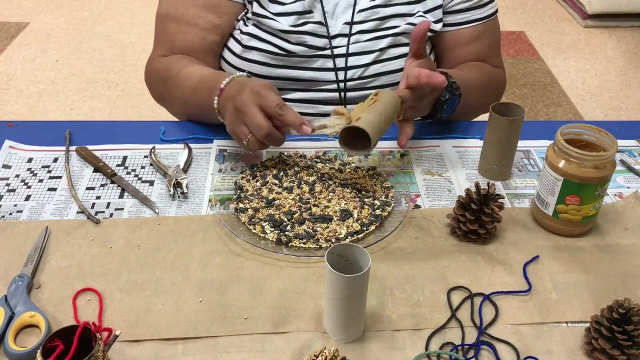 insert the string. So you're going to put one on each side so that will hold the string, And then you can put holes in other areas where we're going to put the stick. And then we're going to cover it with peanut butter. So grab a peanut butter. You're basically going to cover around the tissue roll. You can put quite a bit on there, So it'll. 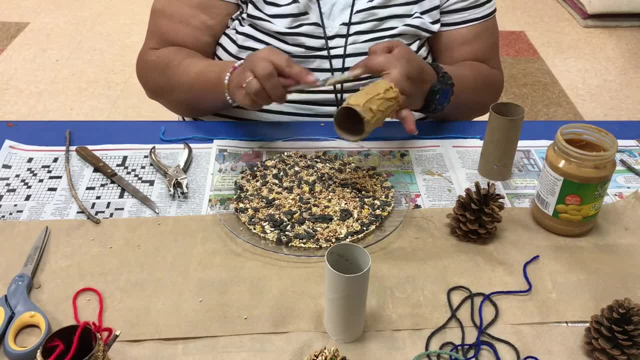 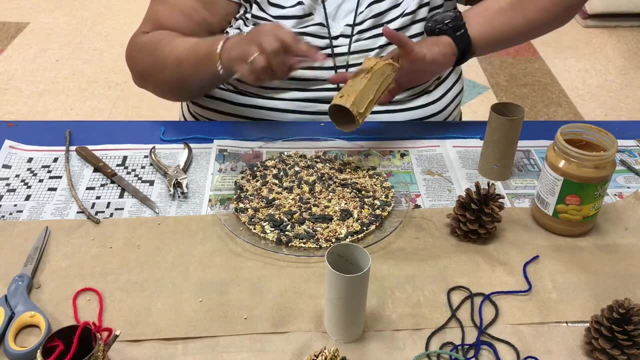 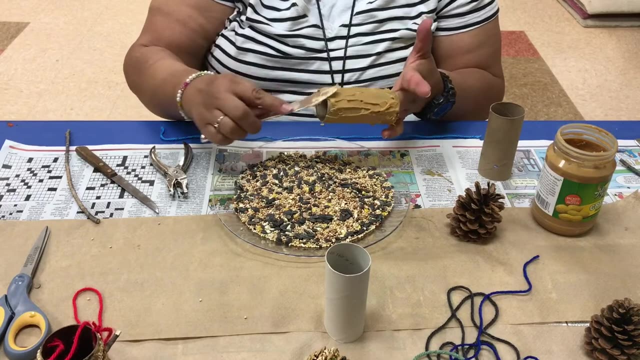 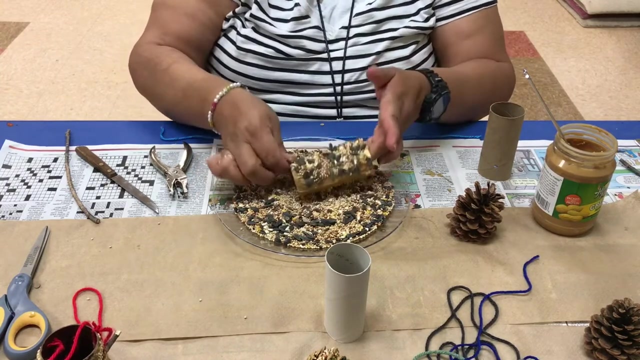 be kind of sticky, But don't worry about that. You can wash your hands And then, once you're done, make sure the whole peanut butter is around the tissue roll. Once you're done, you're going to roll it in the bird feeder and under the seeds and just roll it back and forth. Try to get as much as you can. 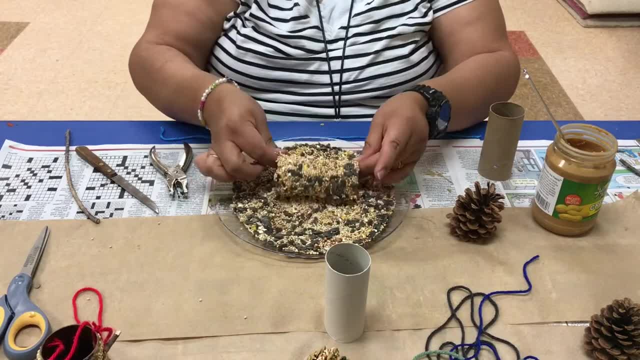 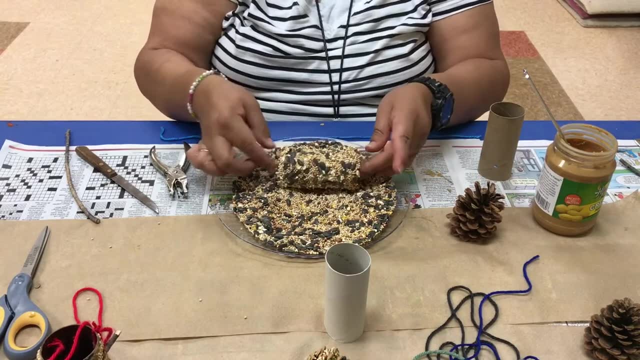 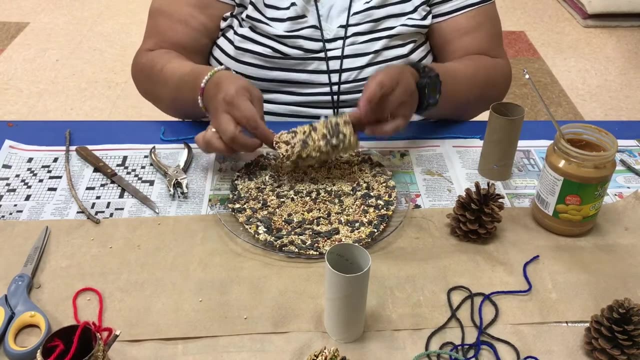 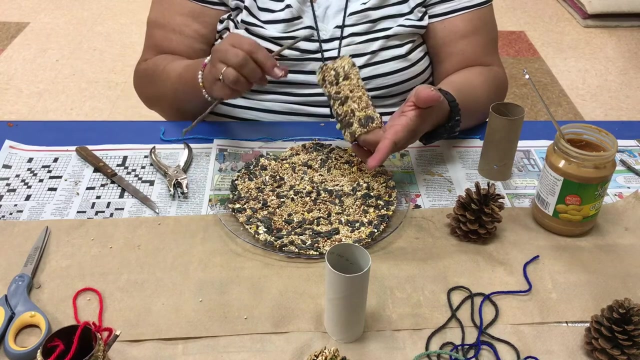 Okay, once you're done, you're going to go ahead and you can let it sit for about an hour or 30 minutes before you can. you want to go ahead and we're going to take some sticks that came off the tree And where we punch holes. you're going to go ahead and find those And we're going to insert. 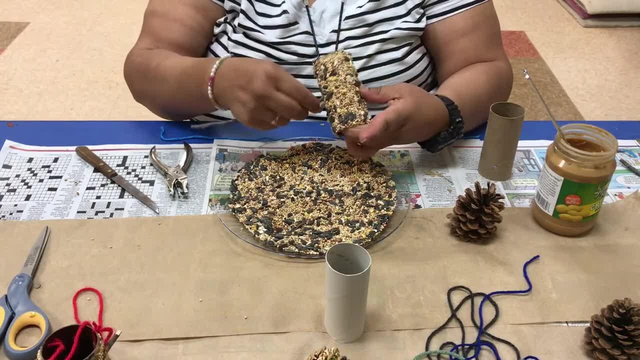 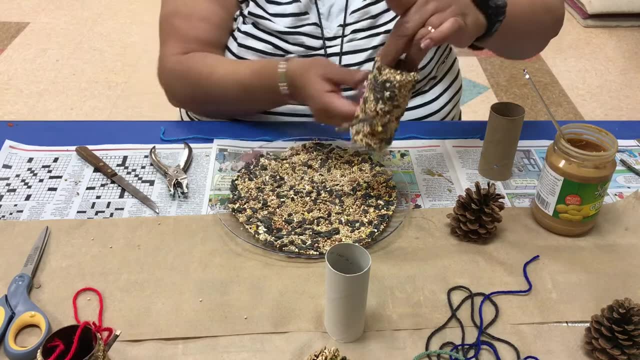 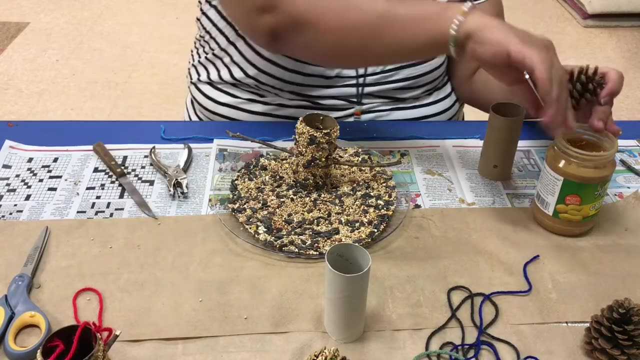 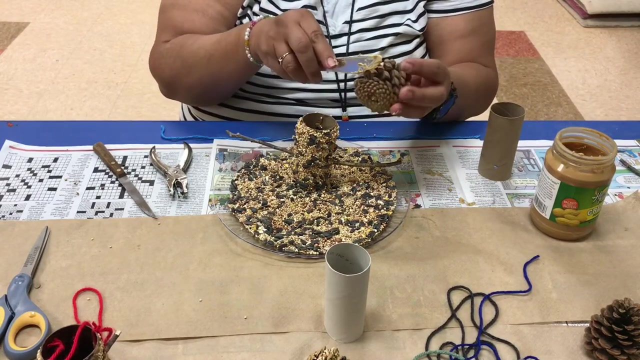 into the. that way, when you hang on a tree- and then we're going to that way- the birds can sit on the sticks. If you use a pine cone, you can also do the same thing. Grab your peanut, peanut butter, and you're just going to put peanut butter, just insert all over the place inside the pine cone. Once you're all done, just same thing. 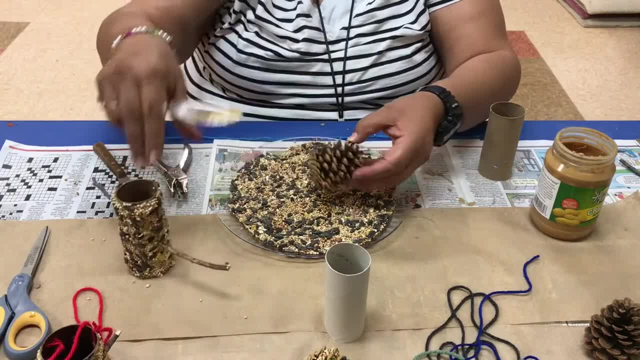 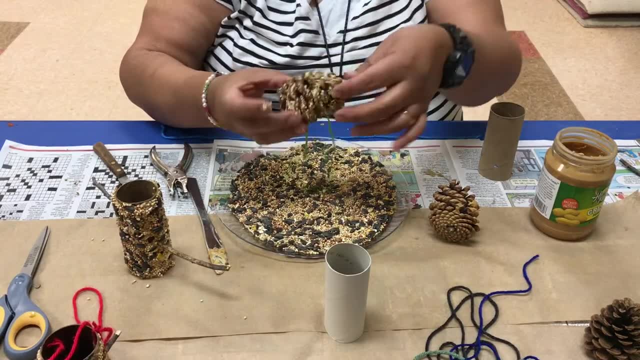 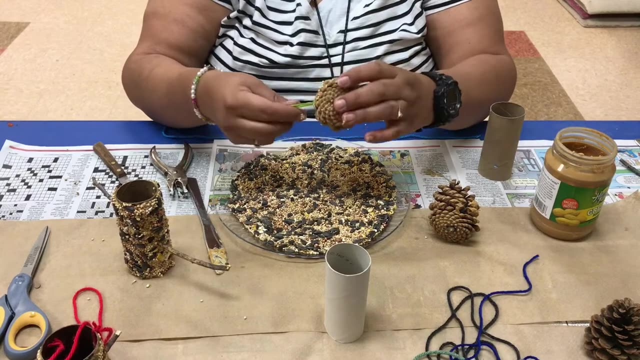 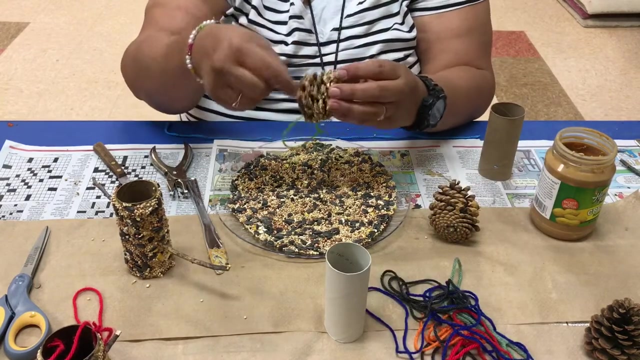 When that's done you can also roll onto the bird feeder and then it's basically going to come up with all of the bird seeds inside the field, inside the gaps of the pine cone. So when that's done you can also let it sit for 30 to an hour. Then, once the seed set in, you can get some yarn and you're just basically going to wrap it around, going way down where you can insert it, and then you can insert it inside.